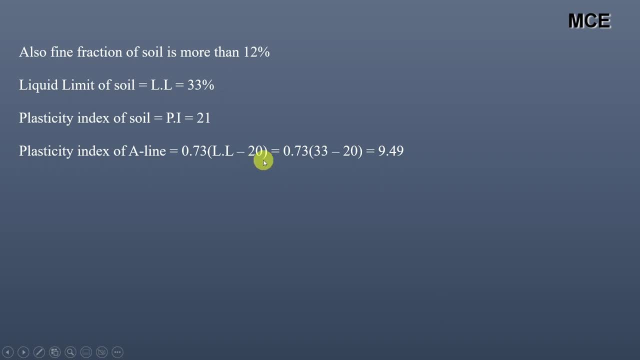 index of A line, which is 0.73 times liquid limit minus 20.. So it will be equal to 9.49.. I can see that PI of the soil is above the PI of A line, So you can say that fine part. 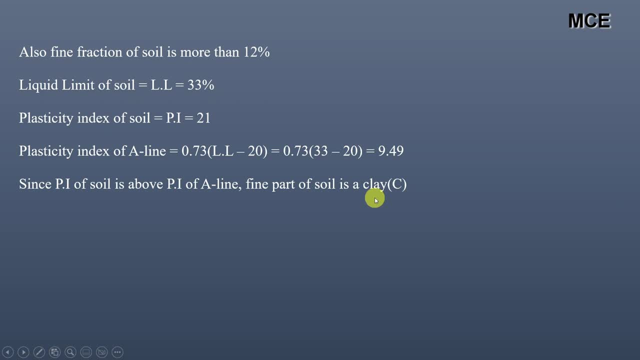 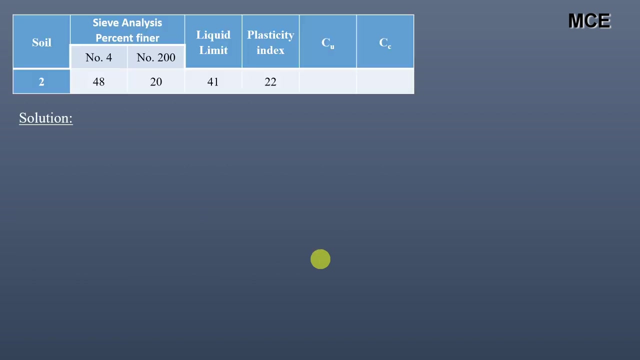 of the soil is clay. That is symbol C will be used. This soil has more than 15% gravel, So it will be included in the group name. So soil will be classified as clay sand with gravel. that is SC. Now for soil 2, I can see that F C- This is 20% C. F is 100-20, which is 80%. 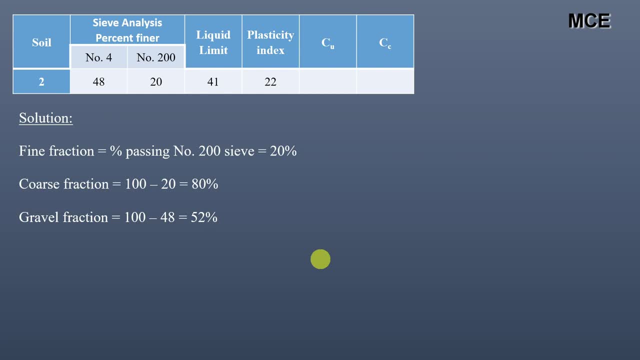 F? C is 100-48,, which is 52%, And F? C is 48-20,, which is 28%. Again for the soil, major portion of soil is coarse fraction and out of this coarse fraction, gravel is. 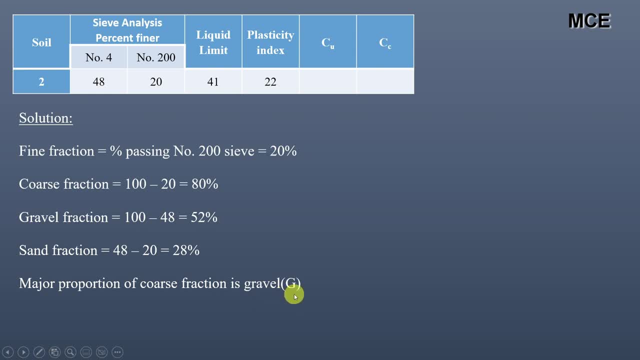 52%, So it's a gravelly soil. Now for soil 2, I can see that P C is 15.. 20% atoms are 6, ama, The în crafts are, so symbol g will be used. fine fraction of this soil is more than 12 percent, so we have to find. 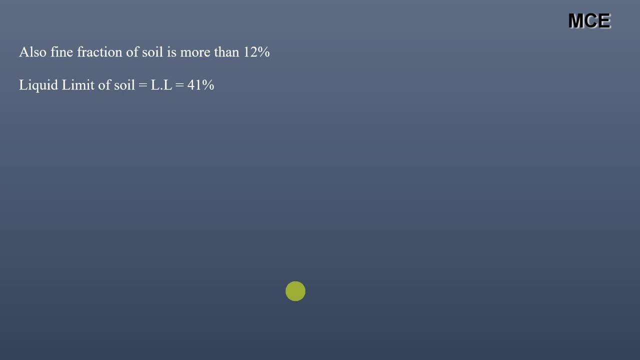 whether it's silt or clay. liquid limit of the soil is 41 percent. plasticity index is 22. plasticity index of a line is 9.03. again, pi of the soil is above the pi of a line, so fine part of the soil. 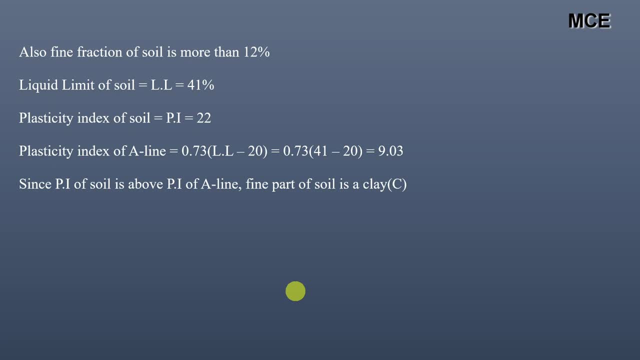 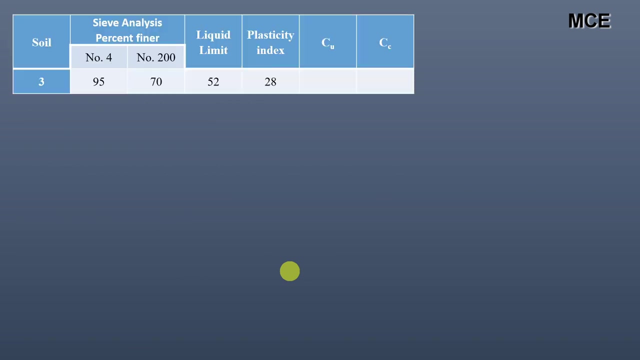 is clay. that is symbol c will be used again. this soil has more than 15 percent sand so it will be included in the group name. so i can say that soil is classified as clay grell with sand, that is. the group symbol will be gc and group name is clay grell with sand. for soil 3 fine fraction is 70. 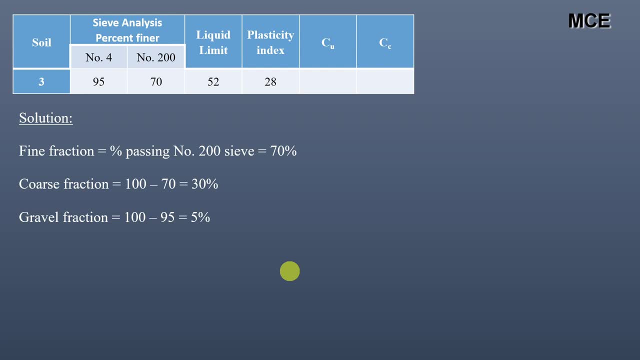 coarse fraction is 30 percent. gravel fraction is 5 percent sand fraction. this is 25 percent. again in this soil we can see the major portion of the soil is fine fraction, which is 70 percent. so it means this is a fine granite soil because more than 50 percent passes c number 200. 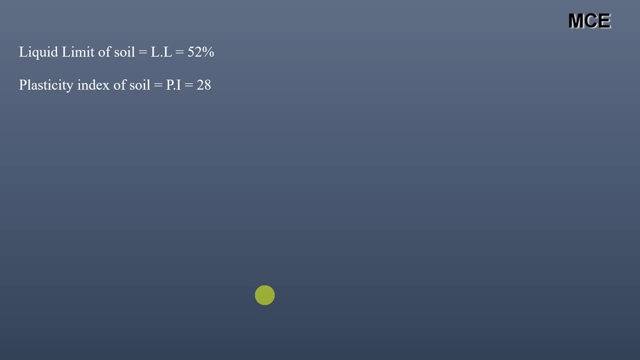 liquid limit of this soil is 52 percent. plasticity index of the soil is 28 and plasticity index of a line is 23.36. for the soil, pi of soil is above pi of a line, so it means fine. part of this soil is clay. liquid limit is greater than 50 percent. 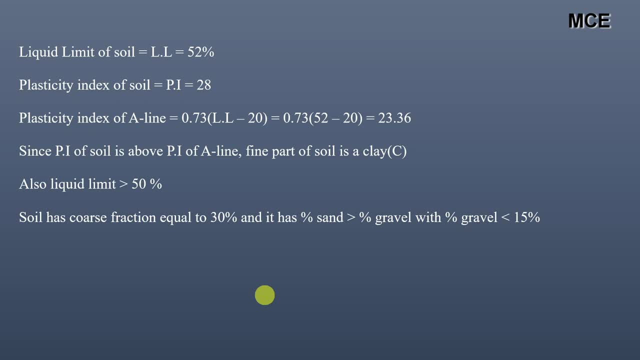 this soil has coarse fraction equal to 30 percent and in this coarse fraction, percentage of sand is less than percentage of gravel and this gravel percentage is less than 15 percent. this coarse fraction will be included in the group name since it is equal, or you can say equal or greater than. 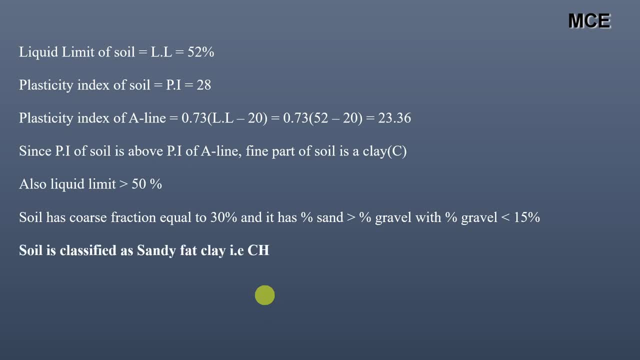 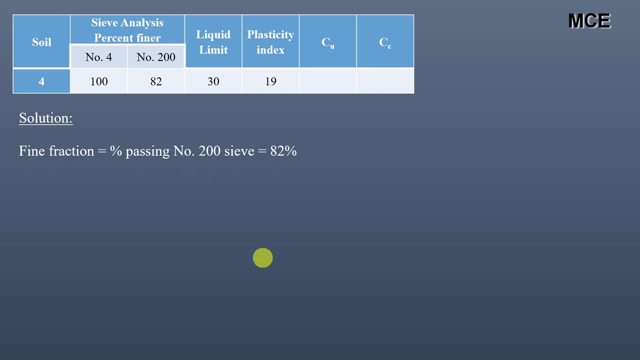 30 percent. it will be written before the group name, so soil will be classified as sandy fat clay. that is the symbol. group symbol will be ch for soil. four is 82 percent. coarse fraction is 18 percent. gravel fraction is zero. sand fraction is 18 percent. 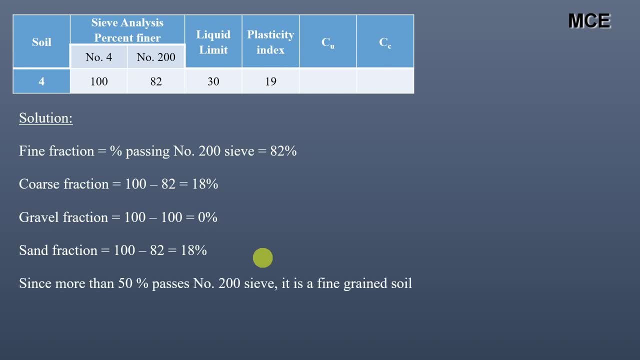 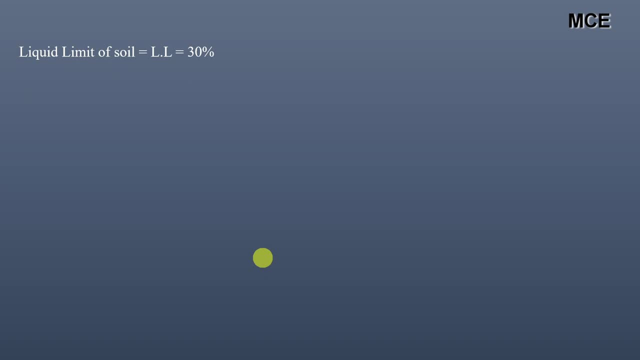 and for the soil more than 50 percent passes the c number 200. so it's a fine granite soil. liquid limit of the soil is 30 percent. plasticity index is 19. pi of a line is 7.3. again, pi of the soil is above pi of a line, so fine, part of the soil is clay. that is symbol c. 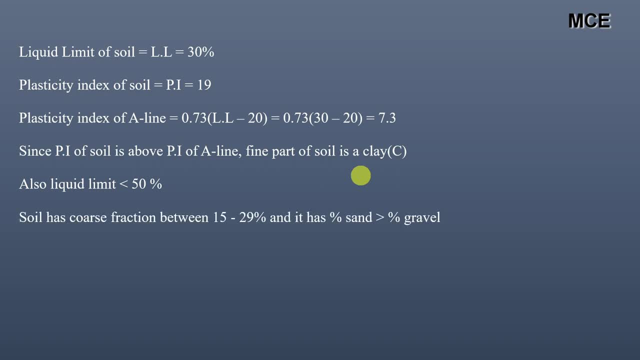 liquid limit is less than 50 percent. this soil has a coarse fraction between 15 to 29 percent and percentage of sand is greater than percentage of gravel. so this coarse fraction- that what type of coarse fraction it is? here it is sandy sand, percentage greater than gravel. so it will be. 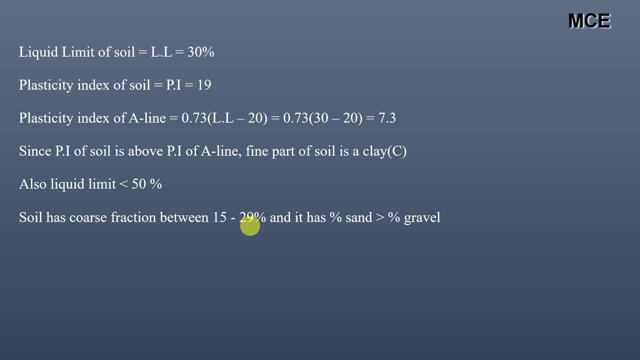 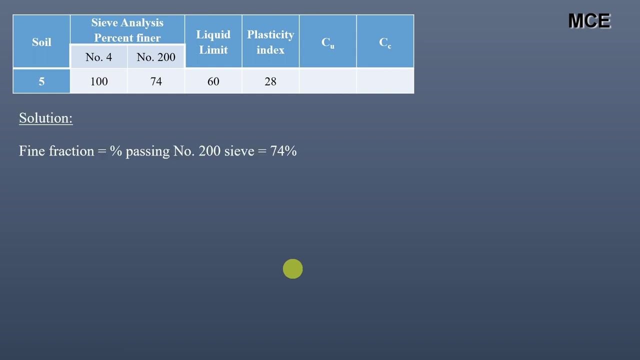 written after the soil, after the group's name, that is. i can classify the soil as lean clay with sand. this coarse fraction is written after the major portion which is the fine fraction which is clay. so grip symbol will be cl. for the soil. five fraction is 74 percent. coarse fraction is 26 percent. 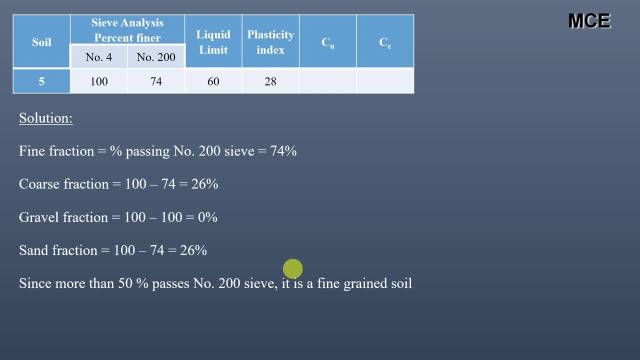 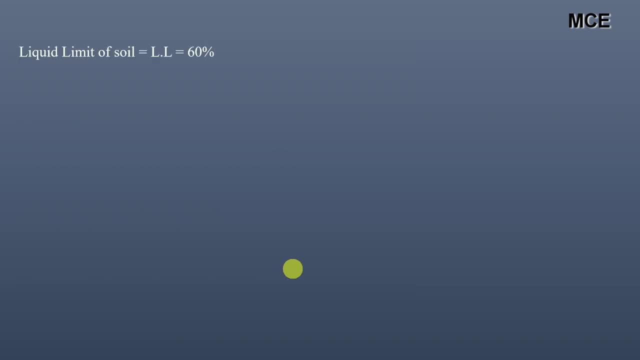 gravel fraction is 0 percent. sand fraction is 26 percent. more than 50 percent passes c number 200, so it's a fine granite soil. liquid limit of this soil is 60 percent plus. the index is 28. pi of a line is 29.2. we can see for the soil. this time the pi of the soil is below the pi of a. 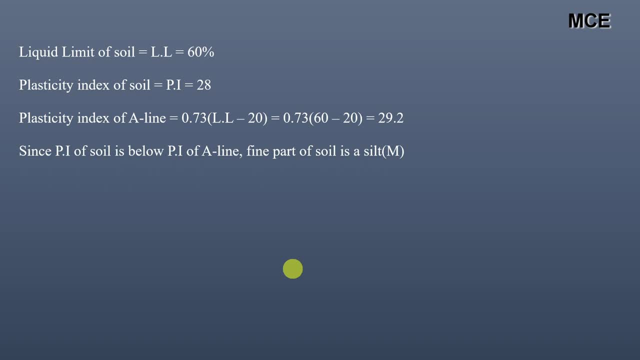 line. it means that the fine part of the soil is a silt. that is symbol m will be used. liquid limit of the soil is 50 percent. soil has a coarse fraction between 15 to 29 percent and percentage of sand is greater than percentage of gravel. so i can write this soil as. classify the soil as. 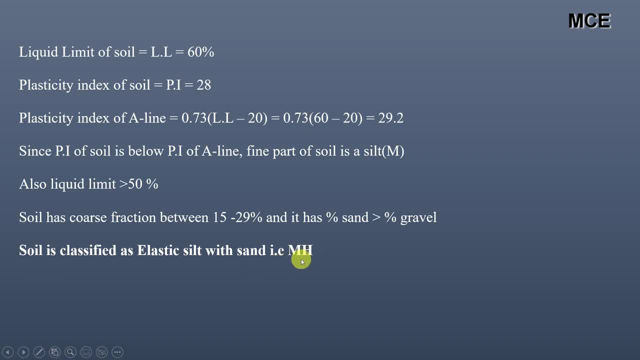 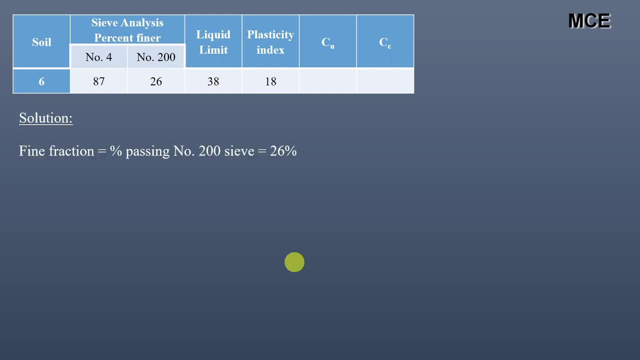 elastic silt with sand and group symbol will be m h for soil 6. fine fraction is 26 percent, coarse fraction is 74 percent, gravel fraction is 13 percent, ayuda fraction is 61 percent and 50 of the coarse fraction it passes sea number 4, so we can say that it's a coarse grain soil. talk about course. 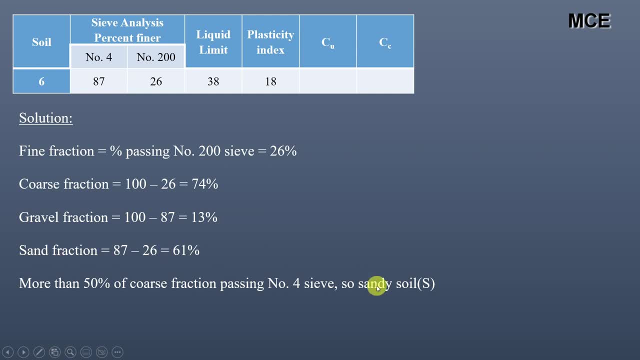 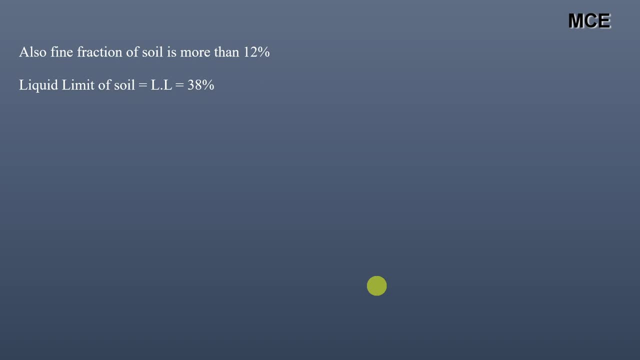 fraction major is sand portion, so we can say it's a sandy soil. fine fraction of this soil is more than 12 percent. it means we have to find out the type of fine fraction. liquid limit of soil is 38 percent. pi of soil is 18, pi of a line is 13.14 and pi of soil is above the pi of a line. it means 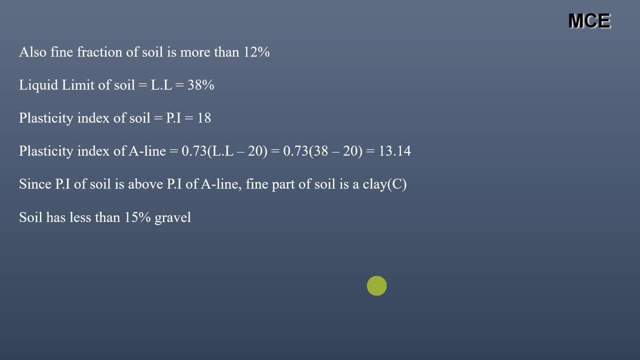 that the fine part of the soil is clay. soil has this is less than 15 percent gravel, so soil will be classified simply as clay sand, that is, the symbol will be sc. if this gravel portion had been more than 15 percent then we should have included this gravel- that is name- with the soil. that is i. 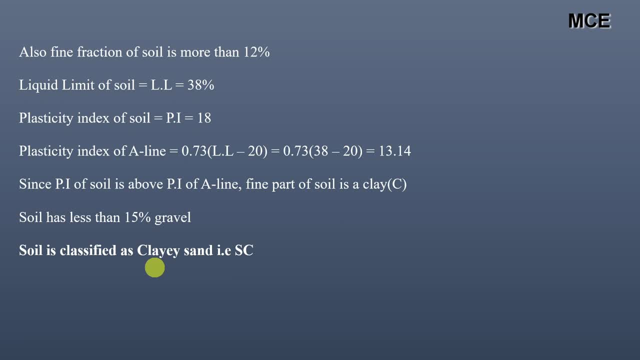 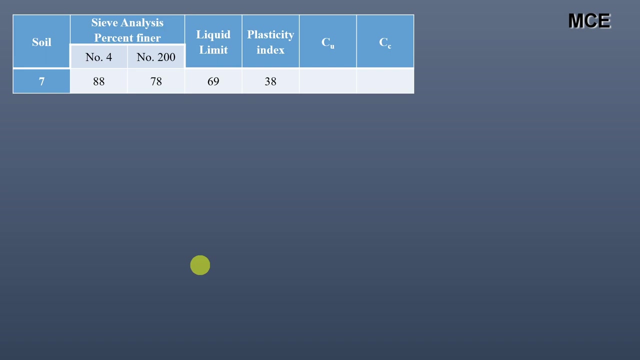 have to write the group name of the soil as clay sand with gravel if it had been more than 15 percent. since it is less than 15 percent, so i don't need to include its name in the group name of the soil. now for soil 7. this has fine fraction equal to 78 percent, coarse fraction: 22 percent. 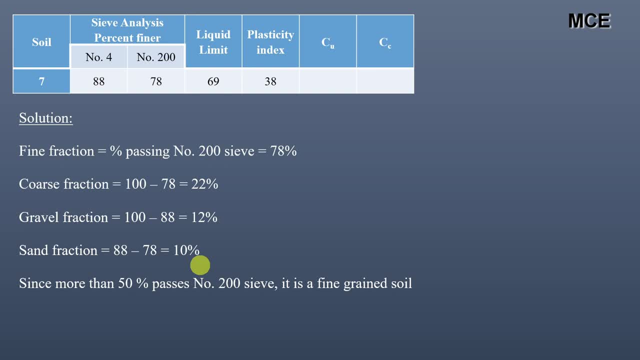 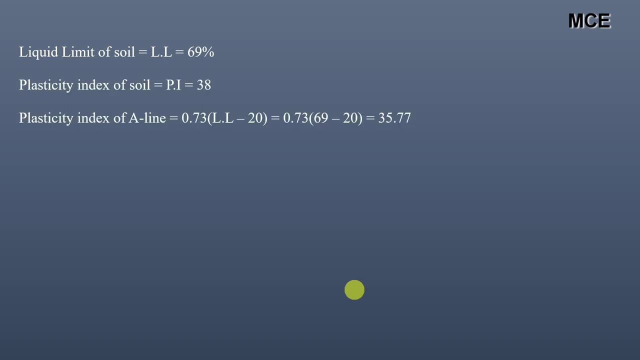 gravel fraction: 12 percent. sand fraction: 10 percent. again we can see that more than 50 percent, that is 78 percent, passes c number two hand. so it is a fine granite soil. liquid limit of the soil is 69 percent. plasticity index is 38 pi of a. 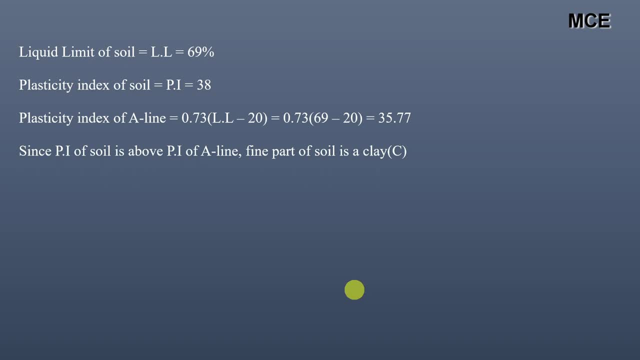 line is 35.77 for the soil. pi of the soil is above the pi of a line, so fine. part of the soil is clay. liquid limit is greater than 50 percent. this soil has a coarse fraction between 15 to 29 percent with the percentage of gravel, with percentage of greater than percentage of sand. 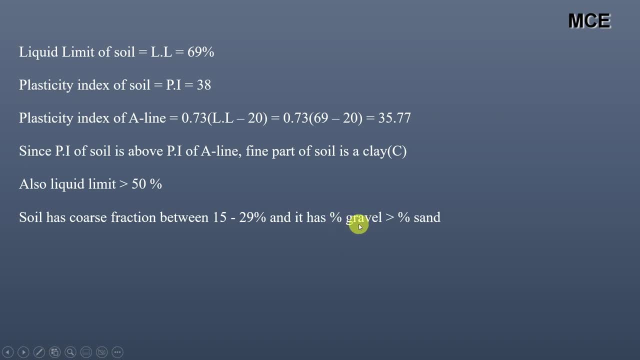 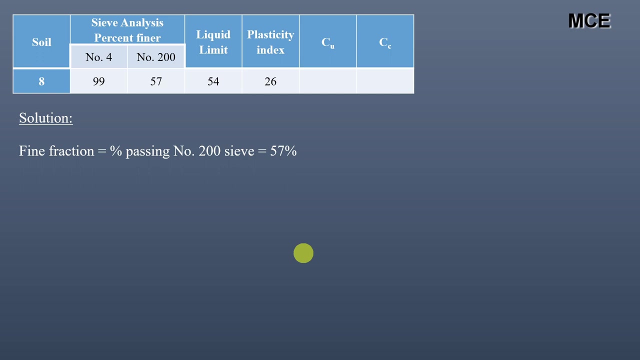 so the name of this gravel will be included in the group name of soil, so soil will be classified as fat clay with gravel that is. the group symbol will be ch for soil 8. fine fraction is 57 percent. coarse fraction is 43 percent. gravel fraction is one. 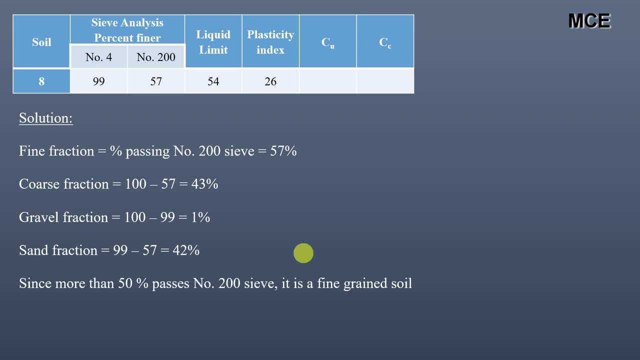 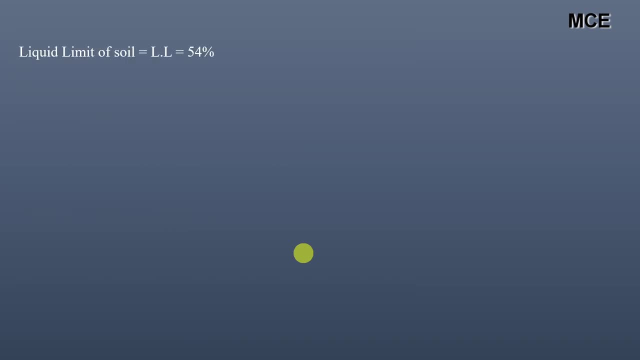 percent. sand fraction is 42 percent and more than 50 percent passes c number 200. so it is a fine granite soil. liquid limit of the soil is 54 percent. plasticity index: pi is 26. plasticity index of a line: this is 24.82. since pi of this soil is above the pi of a line, i can say that fine part. 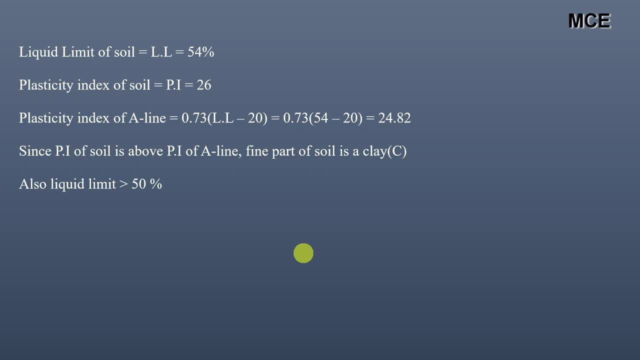 of the soil is clay. also, the liquid limit is greater than 50 percent for this soil is soil. the coarse fraction is more than 30 percent and out of this coarse fraction, sand percentage is greater than gravel percentage, with gravel percentage less than 15 percent. so i can classify. 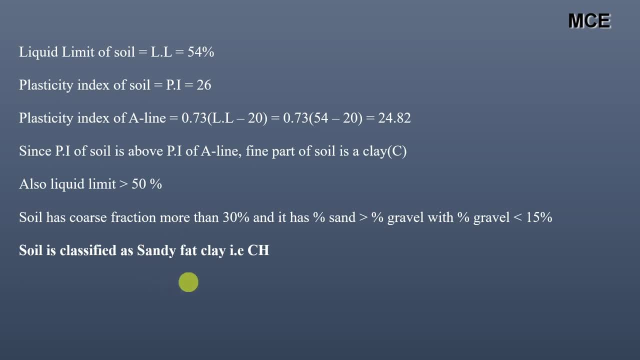 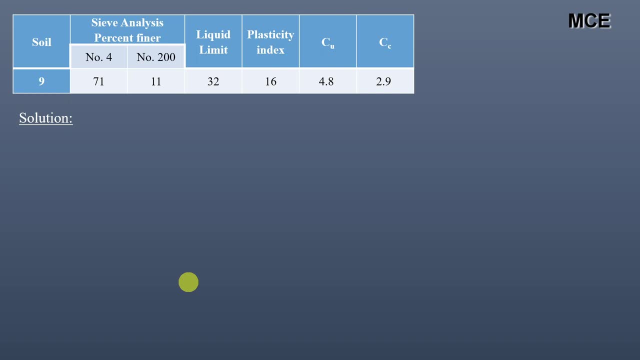 the soil as sandy fat clay, that is. the group symbol will be ch for soil 9. fine fraction is 11 percent, coarse fraction is 89 percent, gravel fraction is 29 percent, sand fraction is 60 percent and 50 percent of the coarse fraction. since this soil, major fraction of the soil is coarse and out of this course i can say that 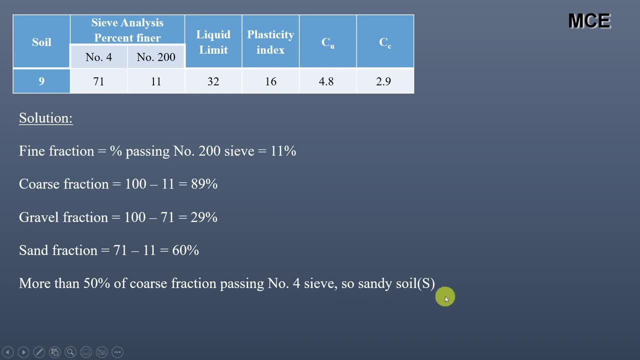 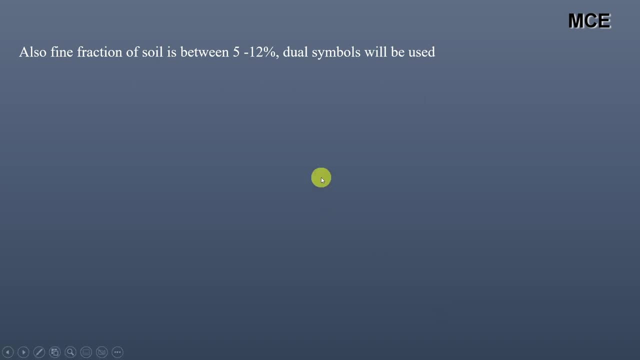 more than 50 percent passes c number 4. so it is a sandy soil, so simple s will be used. fine, fraction of this soil is between 5 to 12 percent. so this means we have to use that dwell symbol. so this means we have to use that dwell symbol. so this means we have to use that dwell symbol. 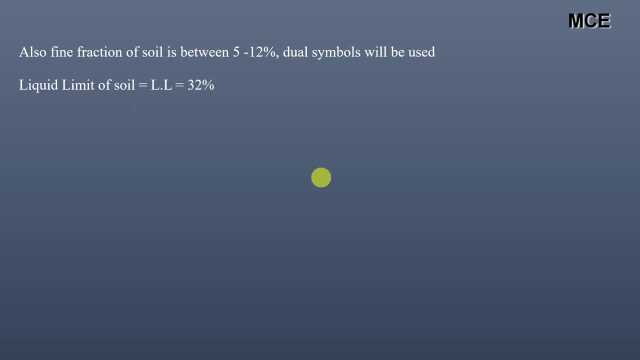 for the soil classification. liquid limit of the soil is 32 percent. plasticity index of the soil is 16.. plasticity index of a line is 8.76. so pi of this soil is above the pi of a line. it means fine part of the soil is clay. 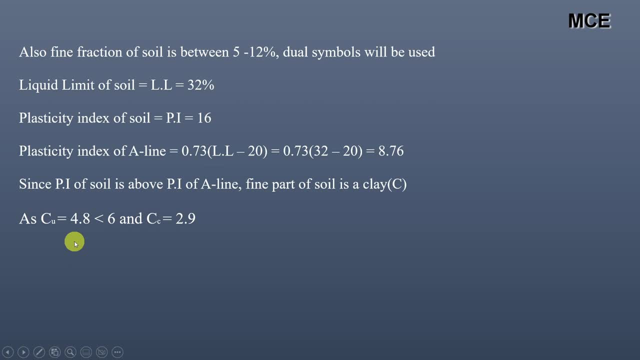 also that is. coefficient of uniformity is 4.8, which is less than 6. coefficient of curvature is 2.9, which is between 2.5 and 2.6, is between 1 to 3.. since coefficient of uniformity is less than 6, so it is a. 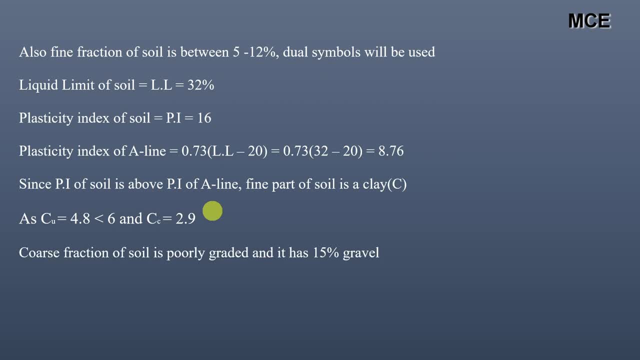 poor graded soil and it has 15 percent grow. so we can classify this soil as poorly graded sand with clay and gravel and the group symbol will be spsc. this is poorly graded because the uniformity coefficient is less than six. for sand it should be greater than six. 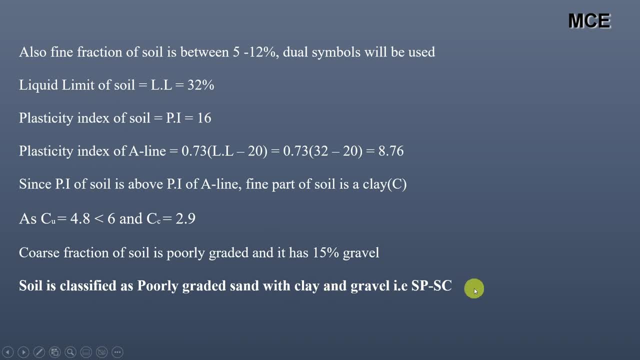 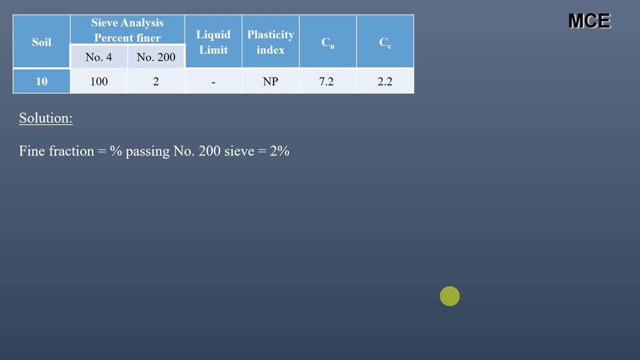 for soil to be well graded. so group symbol of the soil is sp sc. for soil 10 i can see that fine fraction of the soil is two percent. coarse fraction is 98 percent. gravel fraction is zero percent. sand fraction is 98 percent. again for the soil, major portion of the soil is coarse fraction, which is 98 percent. so it means 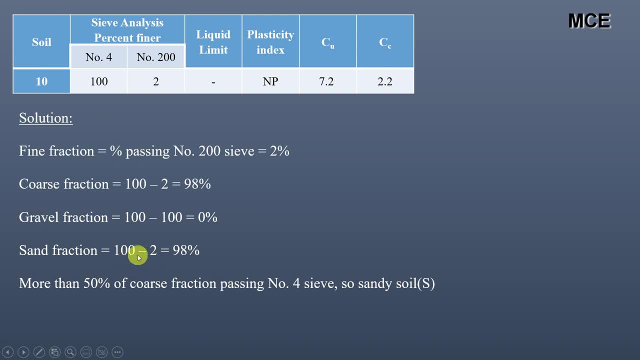 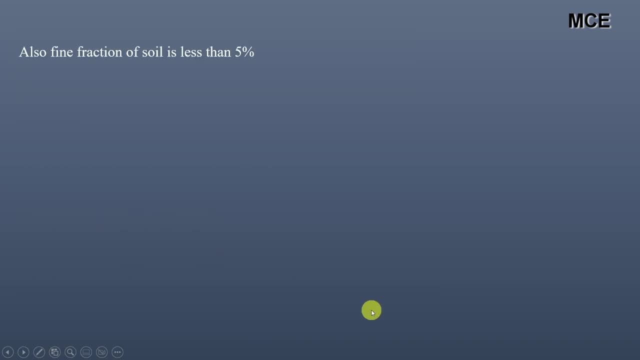 the coarse grain soil and out of this, uh, coarse fraction major is sand, that is 98 percent- is gravel is zero percent. so it is a sandy soil. fine fraction of the soil is less than five percent. so we don't have to find the consistency index of the soil and the soil is non-plastic. we can see for. 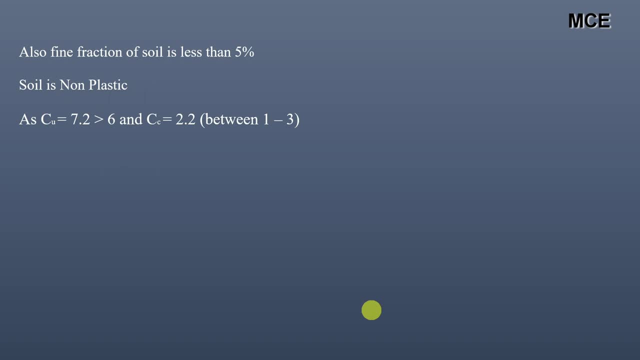 the soil, cu coefficient of uniformity, 7.2, which is greater than six, and coefficient of curvature is 2.2, which is between one to three. it means this soil is well graded. so coarse fraction of soil is well graded, so i can simply classify the soil as well graded sand. that is sw. 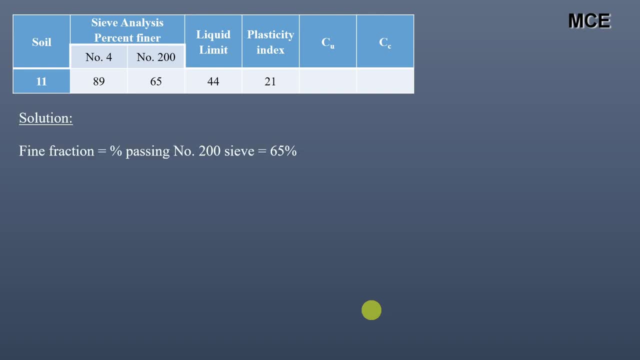 for soil 11. i can see that the fine fraction is 65, coarse fraction is 35 percent. grail fraction is 11 percent. sand fraction is 25, so i can class it s cucumber or so on the nail inichi, so advise that i can count five x xy 5. 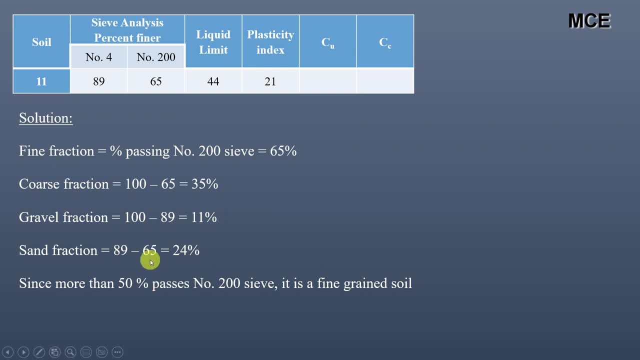 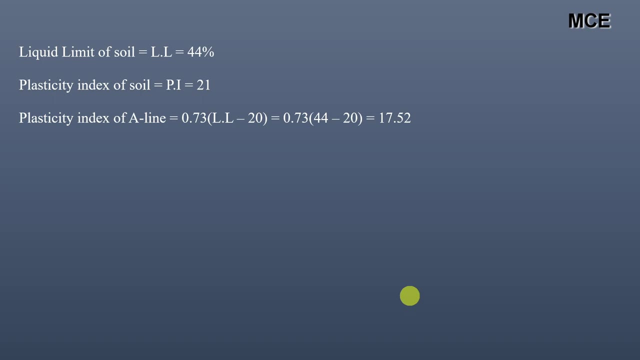 44 percent. for this soil the major portion passes c number 200, that is 65 percent. so we can say it's a fine grained soil. liquid limit of the soil is 44 percent. pi of soil is 21. pi of a line is 17.52. 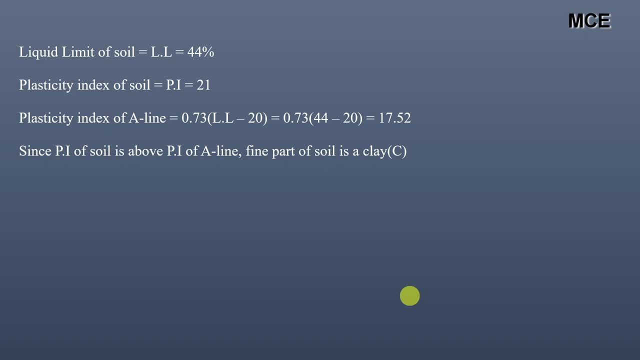 again, for this soil, pi of pi is above the pi of a line, so we can say that fine part of the soil is clay. liquid limit is less than 50 percent and this soil has coarse fraction more than 30 percent, with sand percentage greater than gravel percentage, and this gravel percentage being 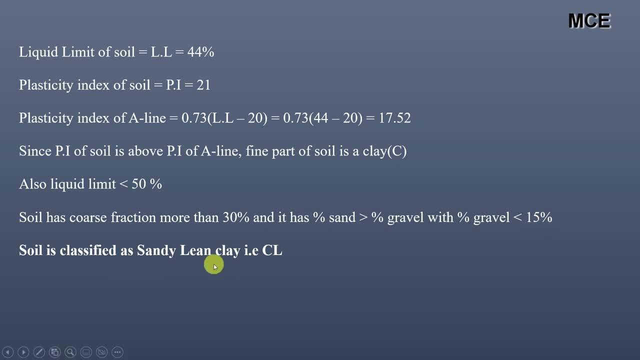 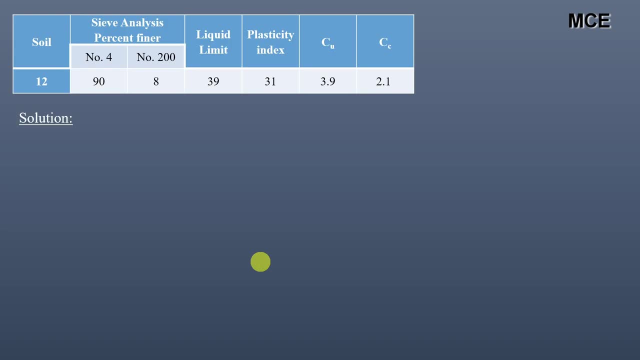 less than 15 percent. so we can classify this soil as sandy lean clay. that is c? l. finally, for soil 12, pine fraction is 8 percent. coarse fraction is 92 percent. gravel fraction is 10 percent. sand fraction is 82 percent for this soil major. 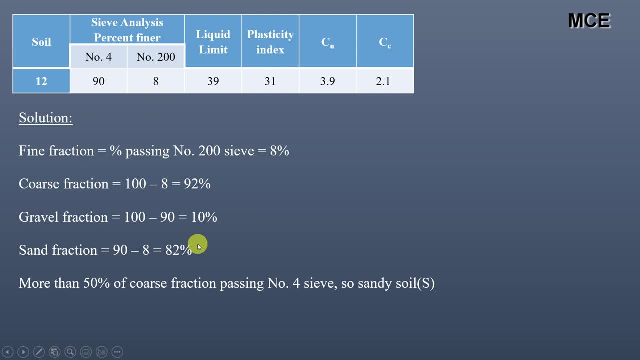 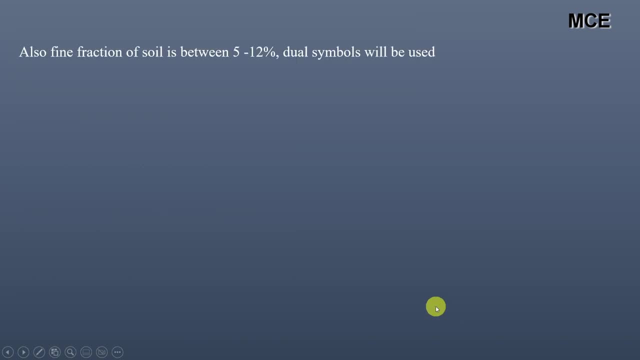 portion is coarse fraction, which is 92 percent, so it's a coarse grained soil. and out of this coarse fraction, sand is 82 percent, so it's a sandy soil. symbol s will be used. fine fraction of the soil is between 5 to 12 percent. again, 12 symbols will be used. first we have to find what type of